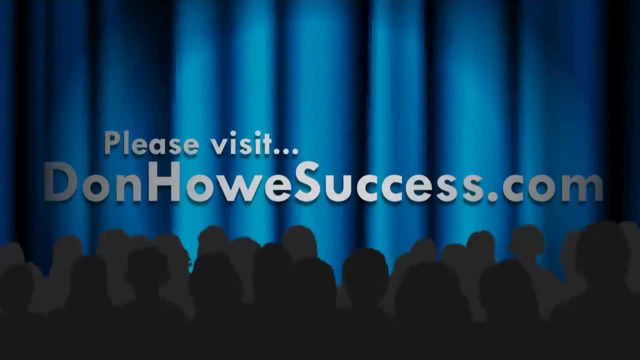 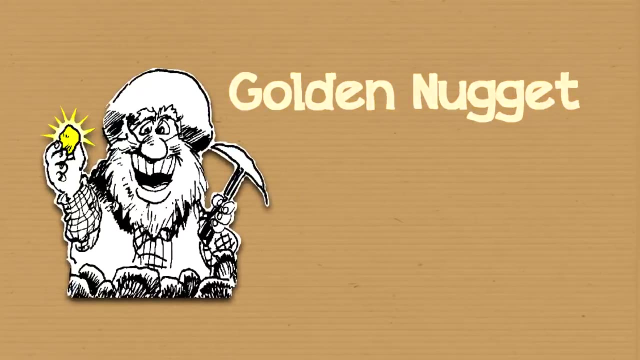 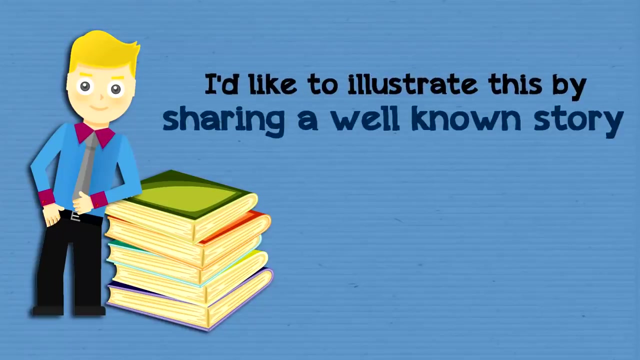 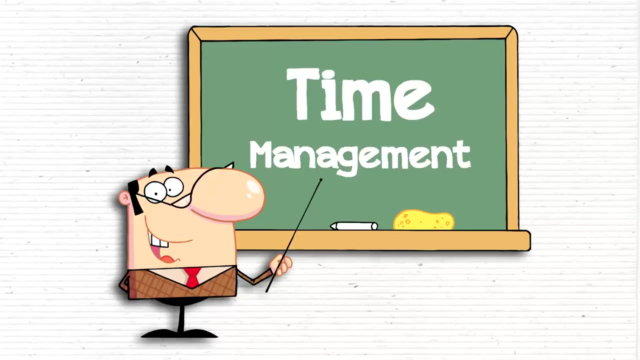 Hi, this is Don Howe, and the topic for this golden nugget is managing your time, and I'd like to illustrate this by sharing a well-known story. Once upon a time, a professor was teaching a class about time management, and the professor set a one-gallon glass jar on the table. 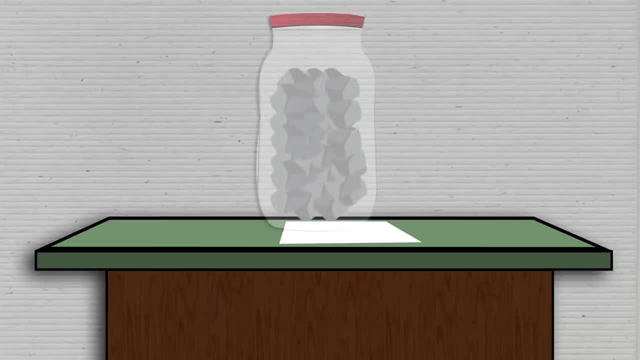 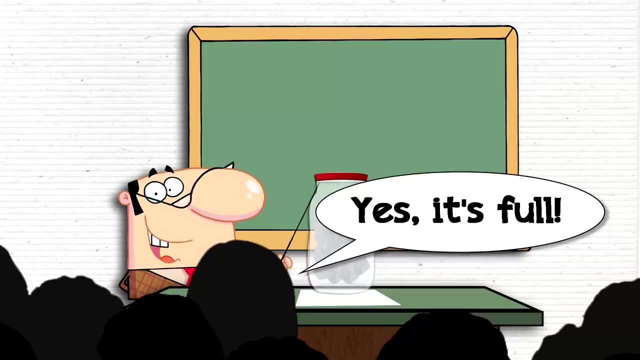 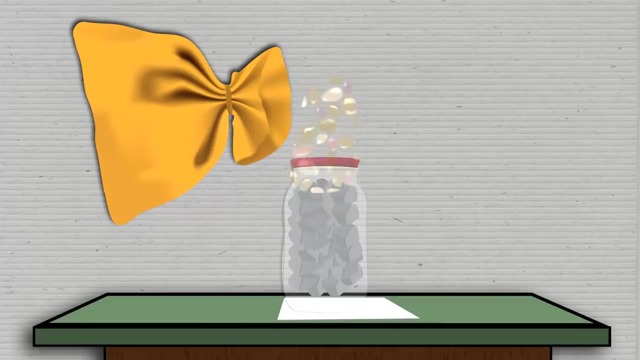 and filled it up with pretty good sized rocks. He then said to the students: is the jar full? They replied yes, it's full. And then he pulled out a bag of pebbles and he poured them into the jar. As he did, he shook the jar so that the pebbles sifted down. 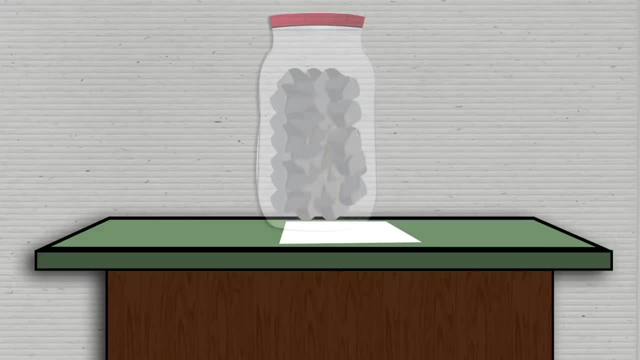 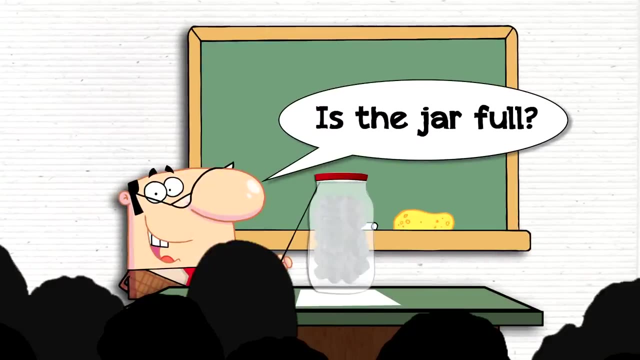 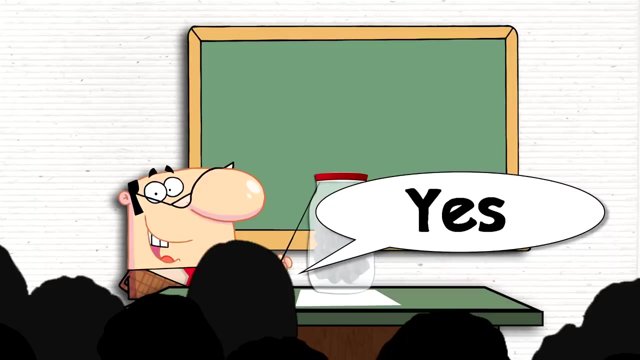 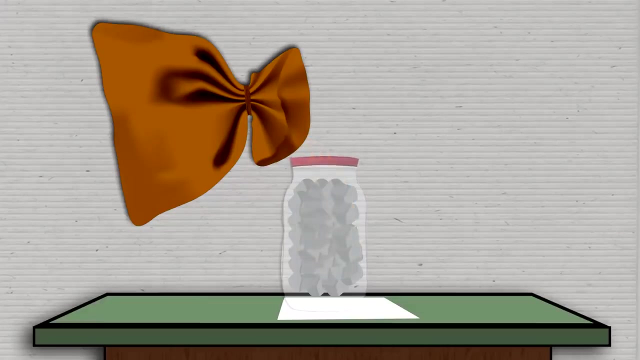 through the holes between the rocks. Eventually the pebbles reached the top of the jar and once again he looked at the class and said: is the jar full? The students cautiously answered yes. And then he pulled out a bag of sand and he did the same thing, pouring and shaking. 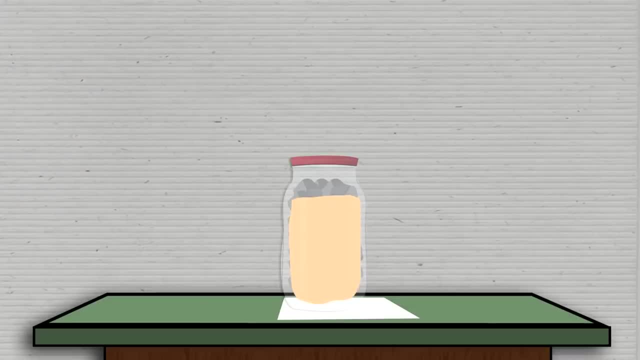 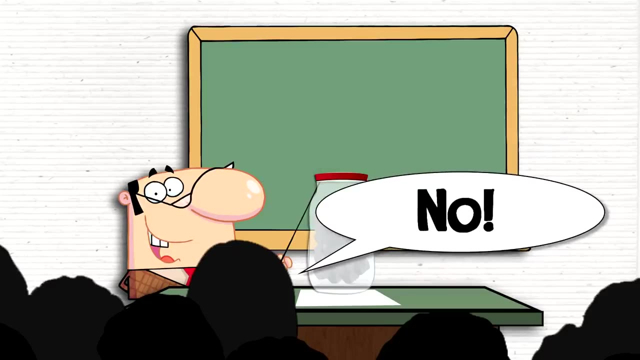 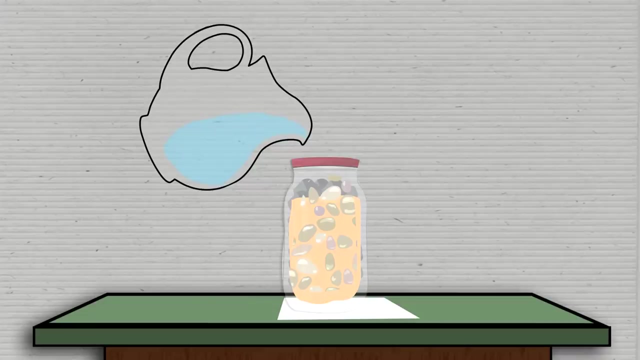 until the sand reached the top of the jar. This time, when he looked at the students and said, is the jar full? They said no. He smiled. He pulled out a pitcher of water. He poured it into the jar until the water. 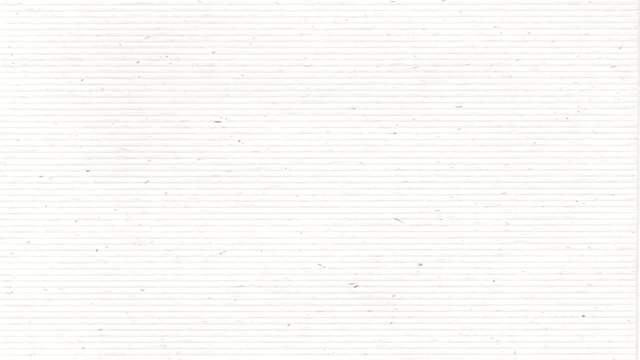 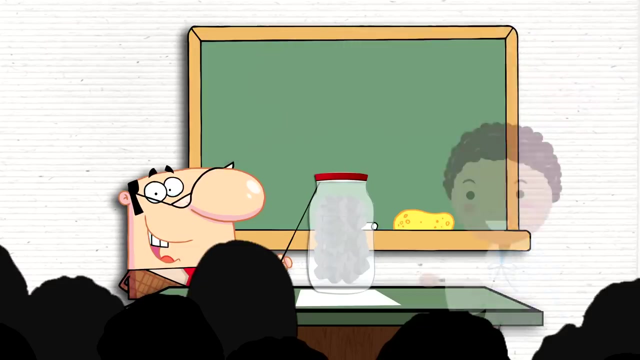 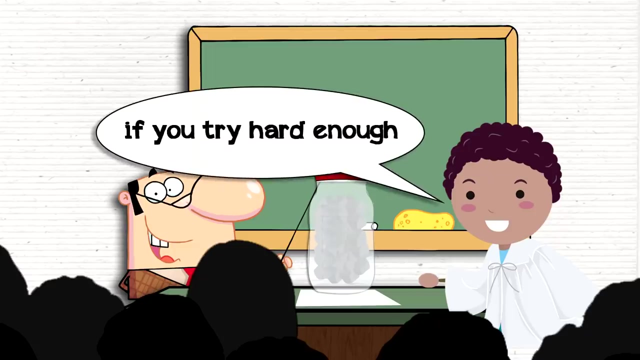 reached the top of the jar And then he looked at the students and he said: what was the point of this illustration? And one young man jumped up and said: I know, No matter how full your schedule is, if you try hard enough, you can always fit some more things. 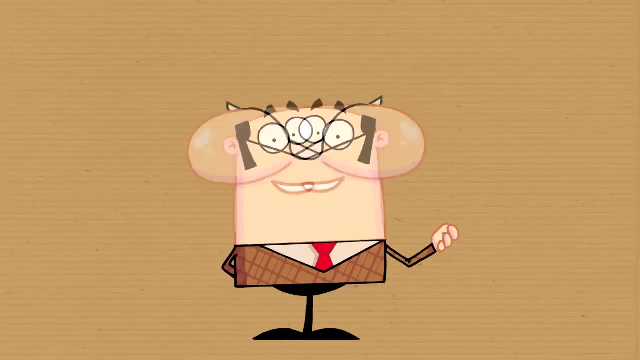 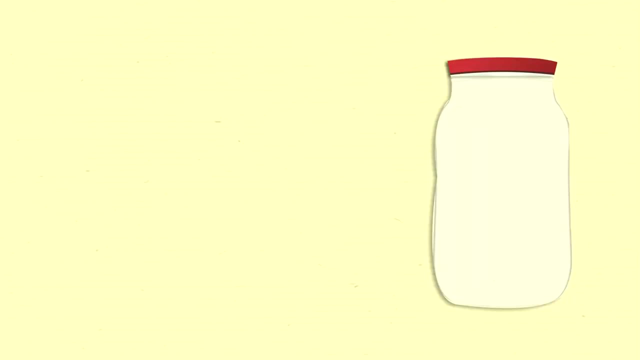 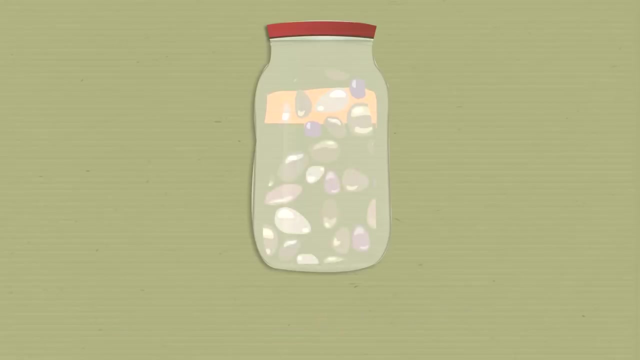 into it. The professor smiled. He shook his head and replied: that's not the point I was trying to illustrate. The point I was trying to illustrate is that if you don't put the big rocks in first, you'll never get them all in. If you fill your jar first with pebbles or sand or water, then